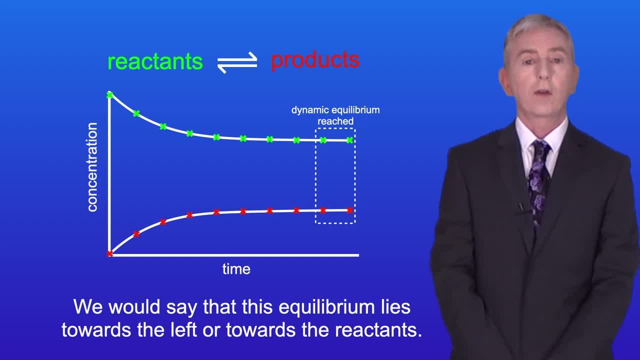 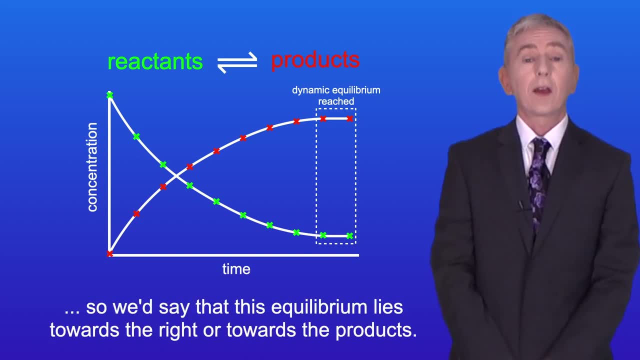 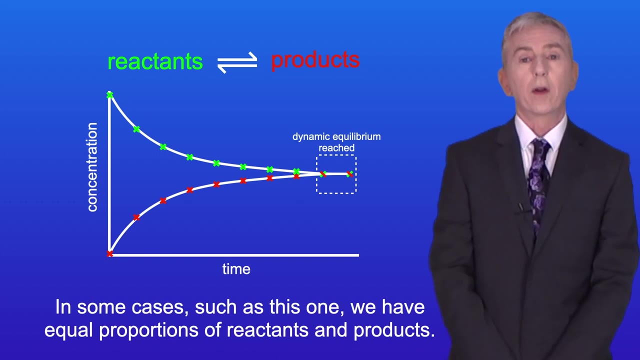 that this equilibrium lies towards the left or towards the reactants. In this equilibrium, we have a greater proportion of products than reactants, So we'd say that this equilibrium lies towards the right or towards the products. In some cases, such as this one, we have equal. 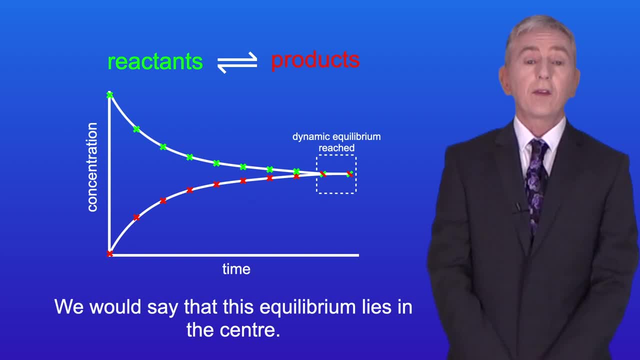 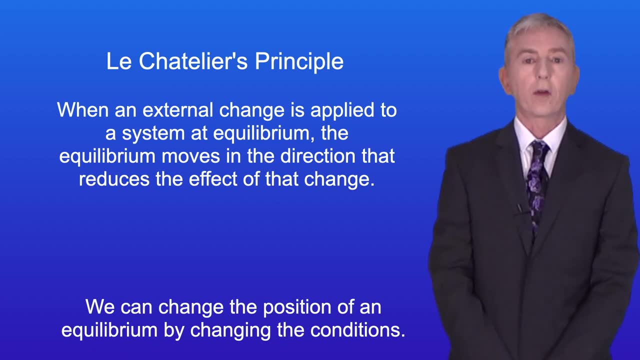 proportions of reactants and products. We would say that this equilibrium lies in the right or towards the products. OK, now we can change the position of an equilibrium by changing the conditions, And the effect of changing the conditions is described by Luchetelier's principle. Luchetelier's principle states that when an external change is applied, 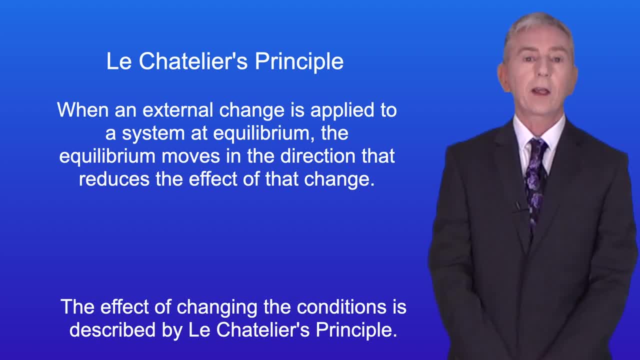 to a system at equilibrium, the equilibrium moves in the direction that reduces the effect of that change. We're going to look at how to apply Luchetelier's principle to changes in concentration, Whereas in later videos we look at the effects of changing the pressure. 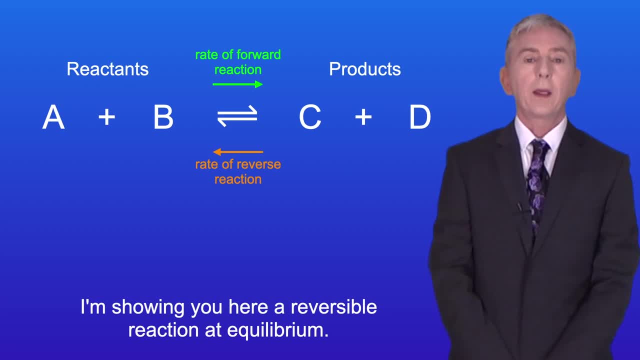 or changing the temperature. I'm showing you here a reversible reaction at equilibrium, And remember that at equilibrium the rates of the forward and reverse reactions are the same. In this reaction, two reactants react to form two products. Imagine that we increase the concentration of reactant A Because we now have more molecules of A. we've 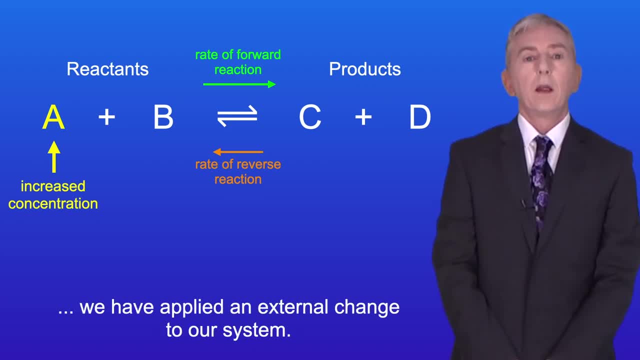 applied an external change to our system. Luchetelier's principle predicts that a reaction at equilibrium will move in the direction that reduces the effect of this change. Because we've increased the concentration of A, the rate of the forward reaction is now greater. 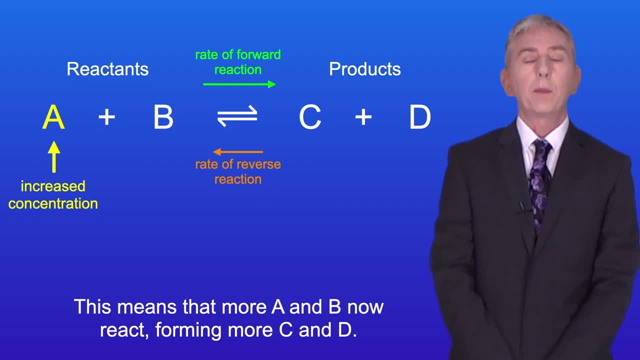 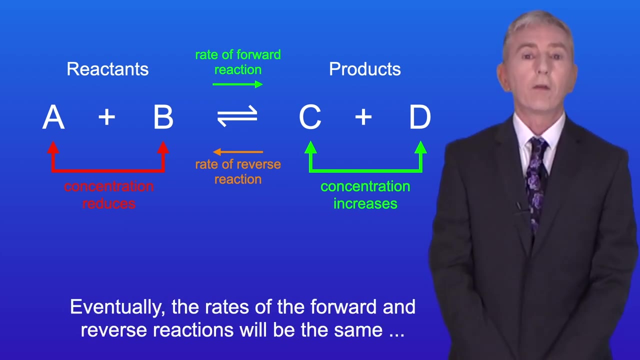 than the reverse reaction. This means that more A and B now react, forming more C and D. So the effect of this is to reduce the concentration of A and B and increase the concentration of C and D. Eventually, the rates of the forward and reverse. 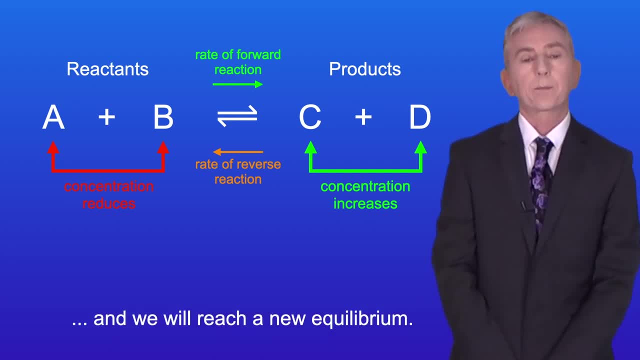 reactions will be the same and we will reach a new equilibrium. So we can see that when we increased the concentration of reactant A, the equilibrium moved to reduce the concentration of A Because we've now formed more products. we can see that the